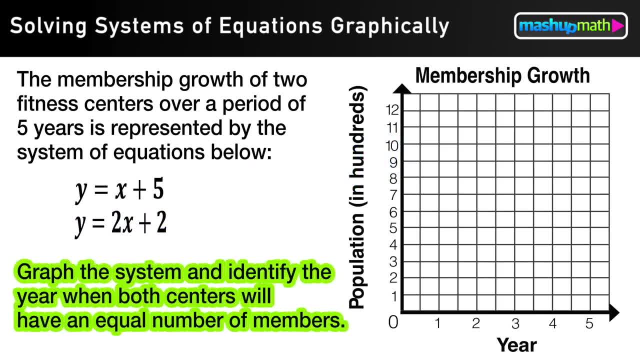 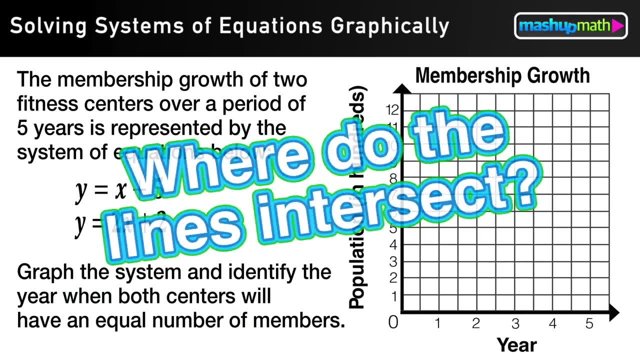 And what we want to do is graph the system and identify the year when both centers will have an equal number of members. So, basically, what we want to know is: when are these two equations going to be the same? at what point? So by graphing them, we can easily find that point. 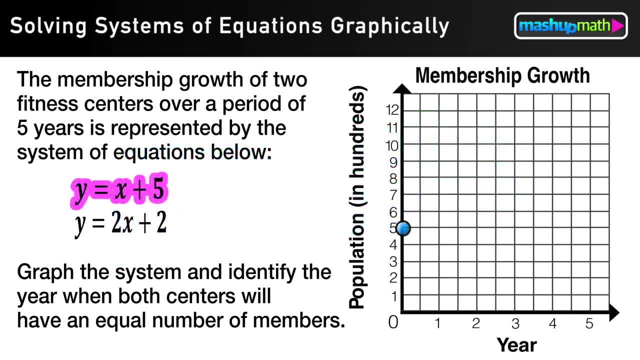 So let's start out by graphing the first equation: y equals x plus 5.. Now our y intercept is 5, so that will be the first point that we plot. And then our slope is 1, so we go up 1, over 1.. 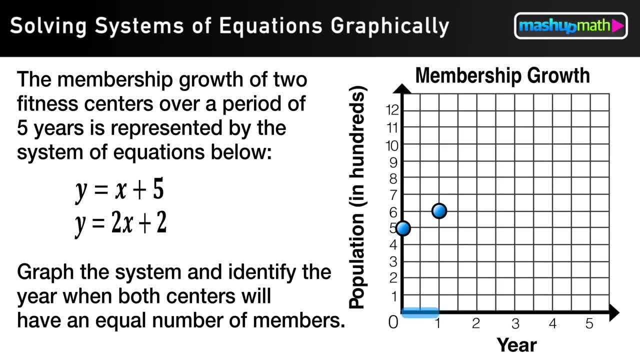 Now notice that on the x axis, two boxes represents 1.. So when I go to the right one, I'm actually going over two boxes And I can continue using this slope to build this line by going up 1, over 1, up 1, over. 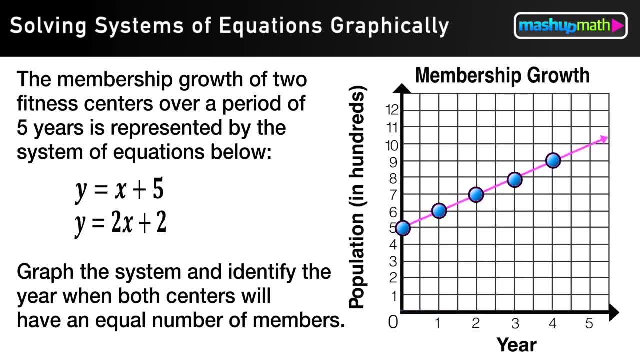 1. And then I can construct the line through the points. Now I can graph the second equation: y equals 2x plus 2.. So now I start at my y intercept of positive 2. And my slope is 2 or 2 over 1.. 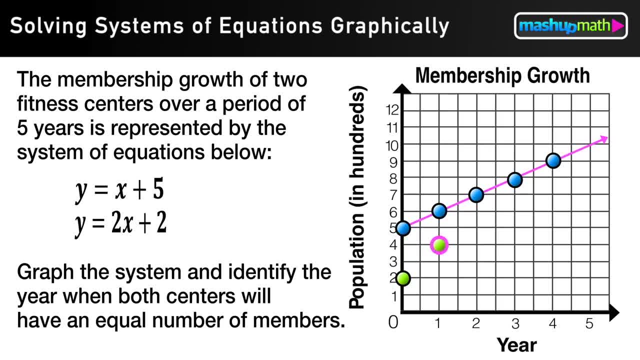 So I go up 2, and over 1.. Again, going over 1 means two boxes here. And I plot my second point And I continue using that slope to graph a few more points And then I can construct my line. 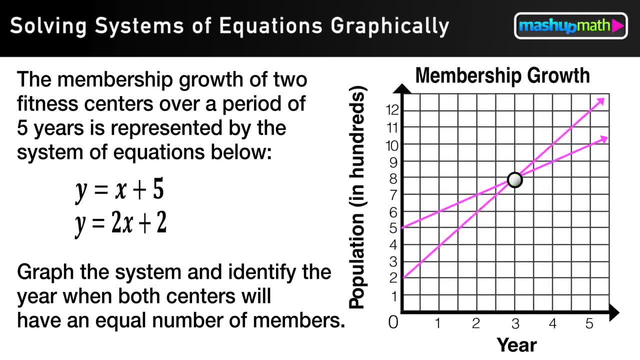 Now I can see where these two equations intersect And I can plot my second point And I continue using that slope to graph a few more points And I find the solution to the system. So remember that we wanted to graph the system, which we just did, and find the year when both systems will have the same number of. 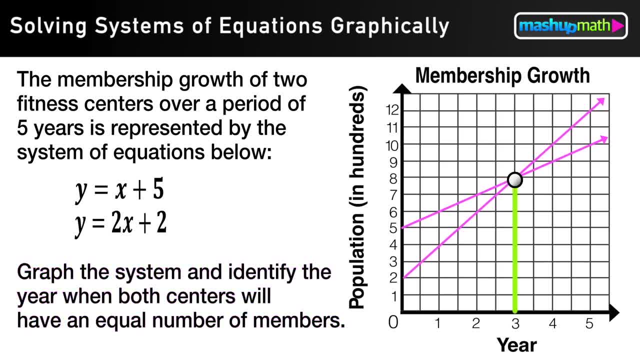 members. So really we want the x value of our intersection point. That's our year, And we can see that in the third year the number of members will be equal. And that's really all there is too. It's just graph the system by graphing each line individually, finding where they intersect. 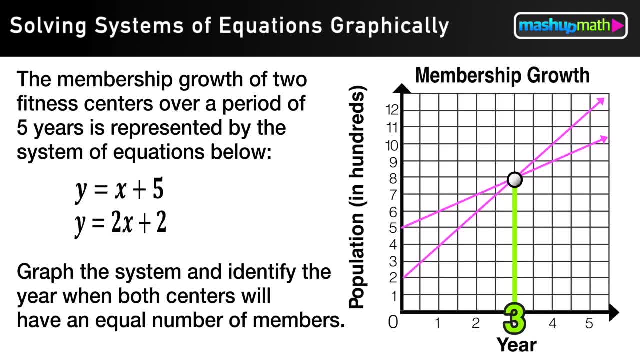 and then checking for the x axis value and you're done. So thanks again, guys. guys, we'll see you next time.